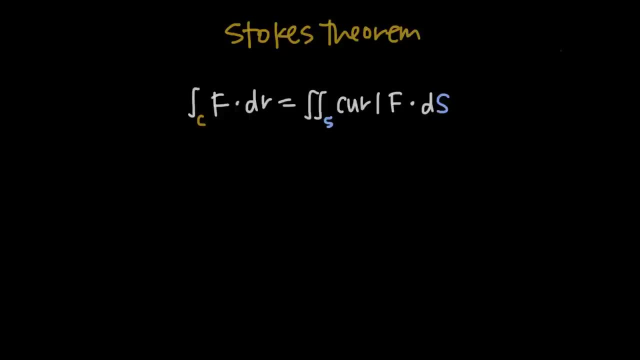 In this video we're going to be talking about Stokes Theorem, And Stokes Theorem is just a higher dimension version of Green's Theorem. So where Green's Theorem only helped us in two dimensions, Stokes Theorem helps us in three dimensions. And the cool thing about 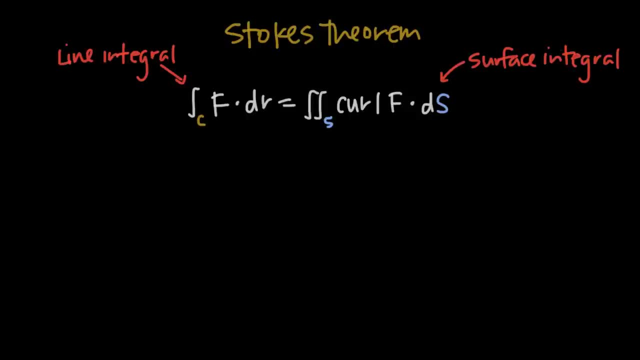 Stokes Theorem is that it relates the line integral to the surface integral. So you'll recognize that you have the line integral on the left side of this Stokes Theorem formula. It's the line integral with the vector function r, the vector field f over the curve c And 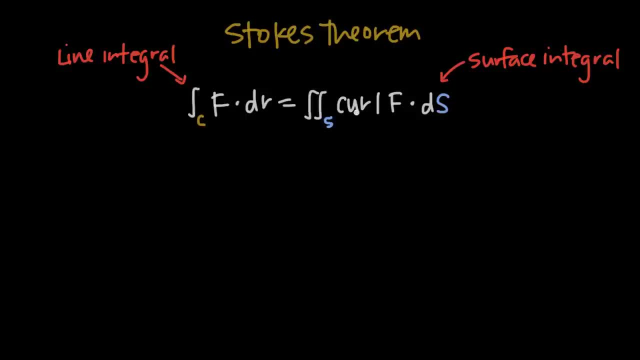 on the right hand side, we've now got a surface integral that includes the curl of the vector field f and the three-dimensional surface s. Now, when it comes to the Stokes Theorem formula, there are a couple things that we need to define. First, we need to say that 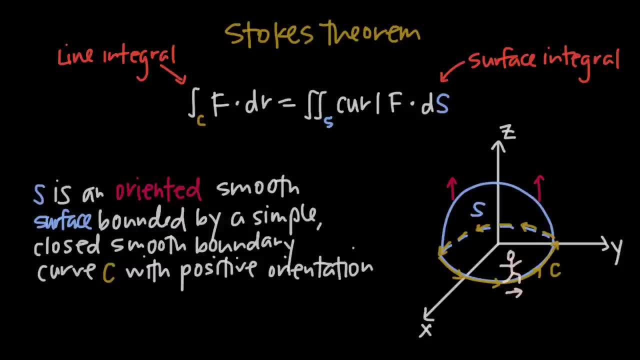 s is an oriented smooth surface. So when we say oriented, we mean that it has a direction in terms of the way it faces. It faces up Or it faces down. Normally we want it to face up, but it really depends on the relationship with the direction of the curve c, which we'll get to in a second. But either way, the surface. 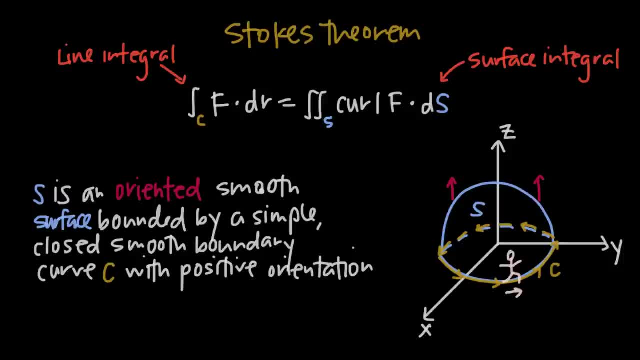 s, it has to have an orientation. So it's an oriented smooth surface that's bounded by a simple, closed, smooth boundary curve c. Notice here that we have the surface s and we have the boundary curve c. Now, in order to use Stokes Theorem, the boundary curve has to have a positive orientation. 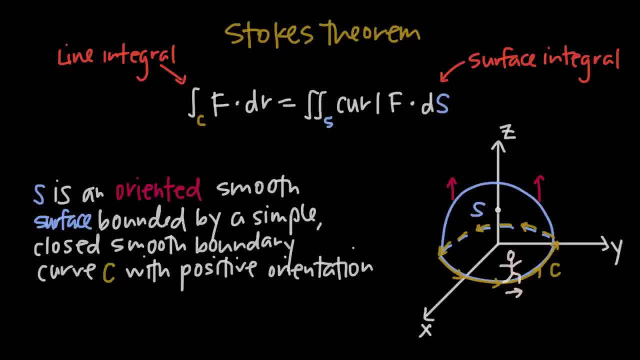 But that relates to the orientation of the surface. Also, Remember that the area between the surface and the boundary curve we want to shift. So what will become of the boundary curve? Well, in this case we're looking at the surface from above of the boundary curve. So in the cz, so in the surface, when we move it clockwise, we still have the closed portion of that boundary curve, But in the looks here disoriented, which is the surface of the curve c, which the corner of the circle is now in content. This is what diretly quarter mice visualizes We can move. 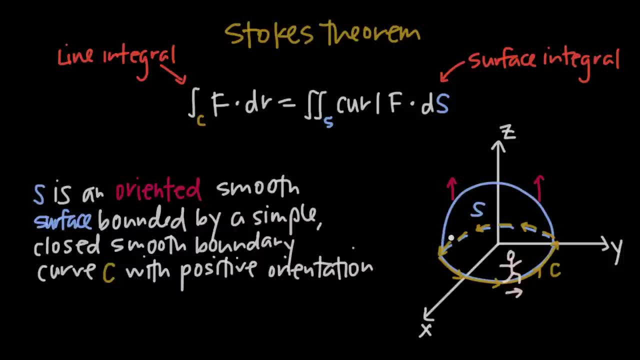 under the surface And the myенно suggest that the globalization of the separating corners counterclockwise direction, because that's what we call a positive orientation for c. If it's oriented clockwise then it's going to be a negative orientation. So we want this positive orientation for c, and one easy way to remember that is to think: 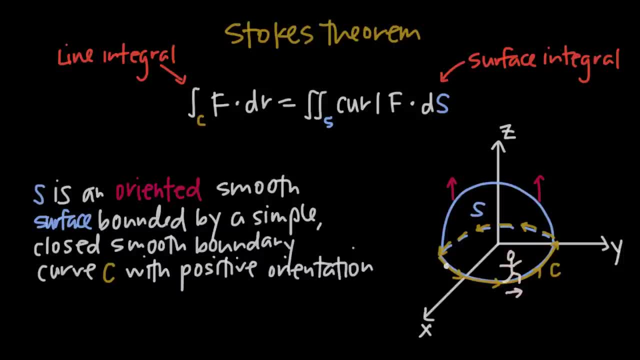 of yourself walking in the direction of the curve c, So we know it has positive orientation, which means we're going in this counterclockwise direction. If we're walking in the direction of the curve c and our head is pointed toward the direction of orientation of the surface, so in this case the surface is pointed up, our head is. 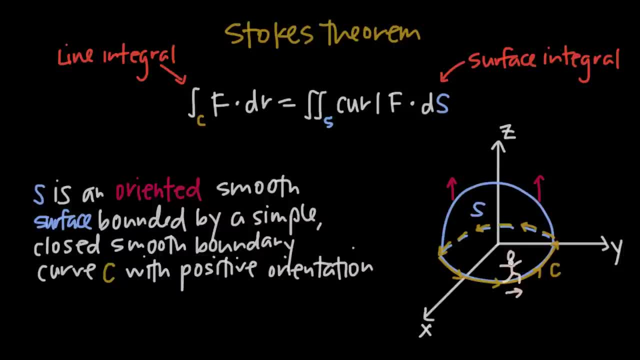 pointed up too, and we're walking in this direction. the surface will always be on our left hand side. If all those conditions are met, if we're able to set up the surface in this way, then we can use Stokes Theorem. 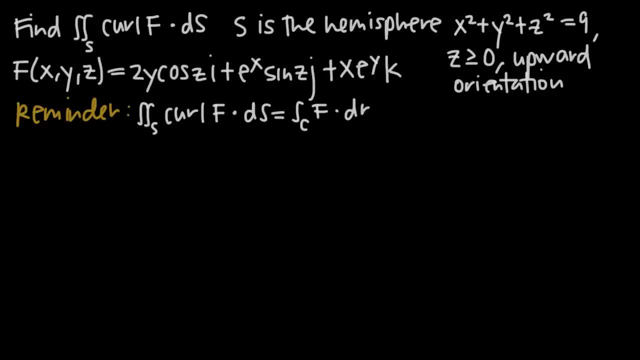 So let's go ahead and do a couple examples Now. the great thing about Stokes Theorem is that, because it relates the line integral over the curve c to the surface integral- and these two things are equal to one another- we can just evaluate Either way. 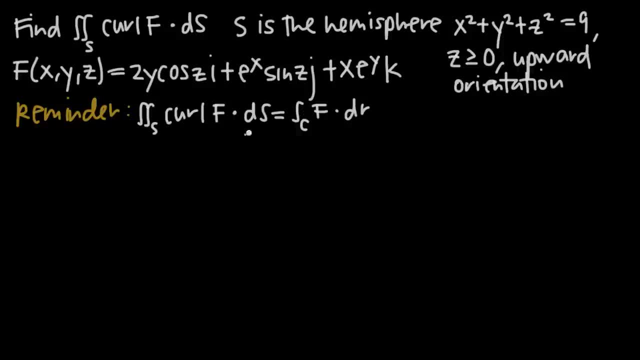 So when you're tackling Stokes Theorem problems, you're either going to be given the information on the left side of this formula and then you'll need to find the value on the right hand side, or you're going to be given the values on the right hand side of the formula. 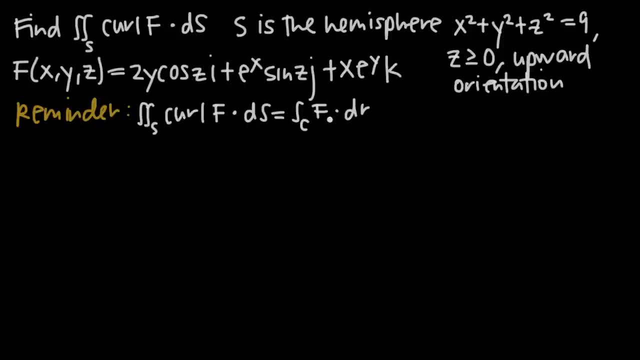 and you'll need to find the values on the left hand side, So we can go either way. Notice, in this case, for this problem, we've been asked to find the value from the left hand side of this formula here. That's a hint to us that the information that we've been given is going to be the information 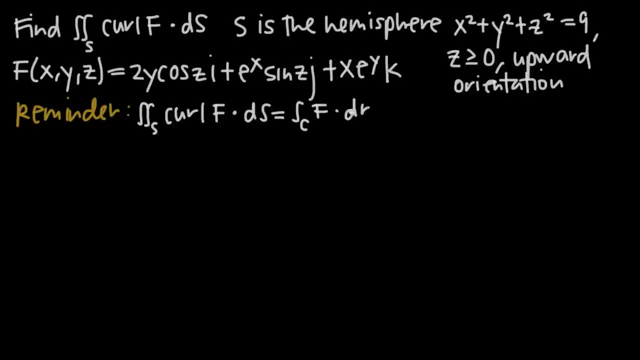 from the right hand side. The first thing we want to do is get an idea of our surface and our boundary curve c. So we've been told that s is the hemisphere, with the equation x squared plus y squared plus z squared equals nine, where z is greater than or equal to zero and the surface has. 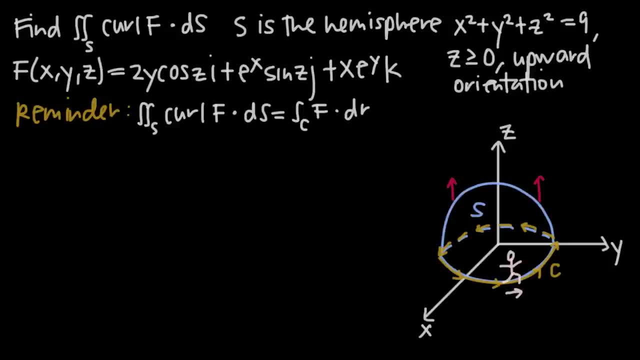 an upward orientation. So, as a matter of fact, that is just about what we drew before. We have the hemisphere that's sitting above the plane. z equals zero, So it's sitting right on top of the xy coordinate plane. It's just the upper half of the sphere. 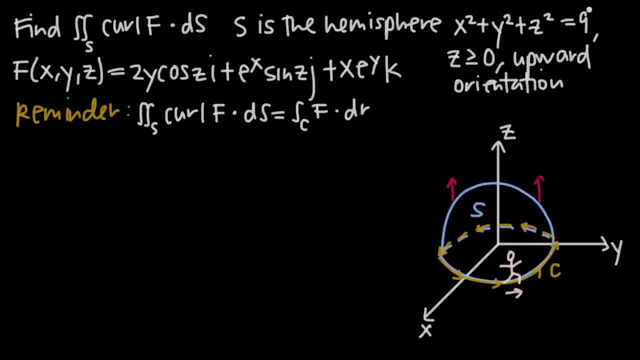 And we know we've got this formula for the sphere, So that's obviously the sphere with radius three. The key, then, is to find this boundary curve c. Well, c runs all along the bottom of the hemisphere, because we're saying that the surface is defined. 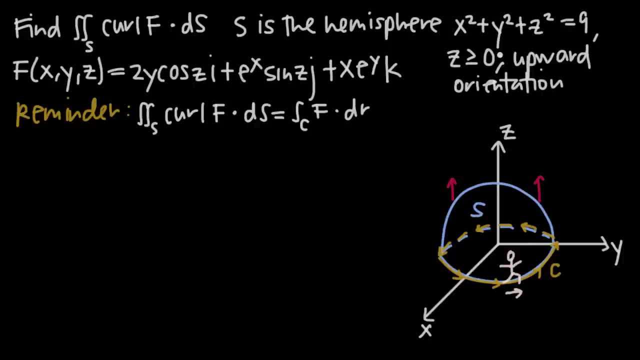 by this equation but cut off at the plane z equals zero. That means that the curve c is going to run along that plane z equals zero along the edges here of the hemisphere and create the boundary for it. So if we want the curve c, what we need to do is plug z equals zero into this equation. 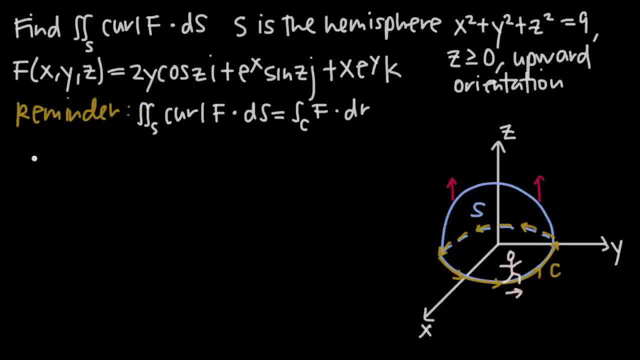 here, And when we do that, we're just going to drop this z squared term and we can say that c is given by x squared plus y squared equals nine when z is equal to zero. Now, remember, we are looking for the information from the right side of this Stokes' theorem. 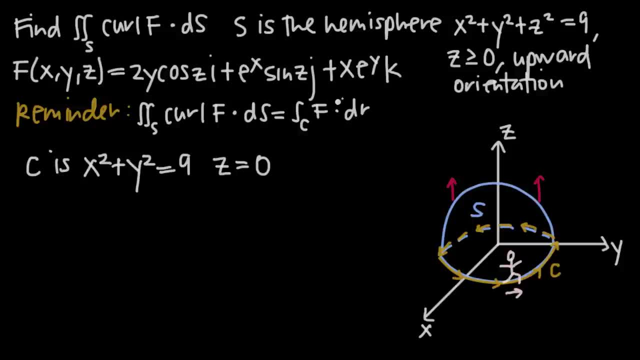 formula. So we just looked at the curve c. But remember, on the right hand side here this dr r is the vector function, which means we want to parametrize this so we can get it in terms of a vector function, Because x squared plus y squared equals nine, is a circle with radius three and that makes 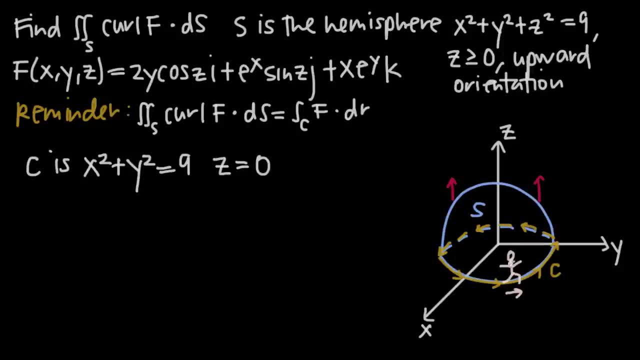 sense, because c here is just the circle centered at the origin in the xy plane, at z equals zero, with a radius of three. That means we can parametrize this as the vector function r of t is equal to. and then, because it's a circle, we always do the radius times cosine. 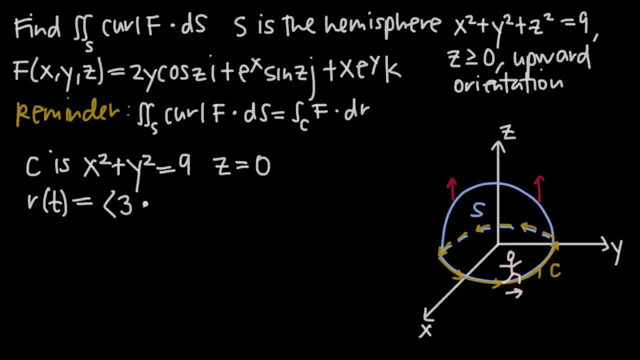 That means we can parametrize this as the vector function r of t is equal to. and then, because it's a circle, we always do the radius times cosine t for x, so three cosine t For y. we do the radius times sine t, so three sine t, and then we already have a value z. 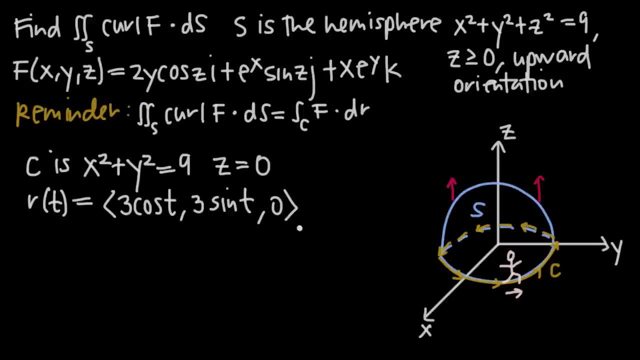 equals zero. so we get z equals zero there. Now, because we've got dr here, we're always going to need to find the derivative of the vector function, so we can go ahead and do that right away, since we're here. So the derivative: when we take the derivative of three cosine t, we get nine times cosine t. 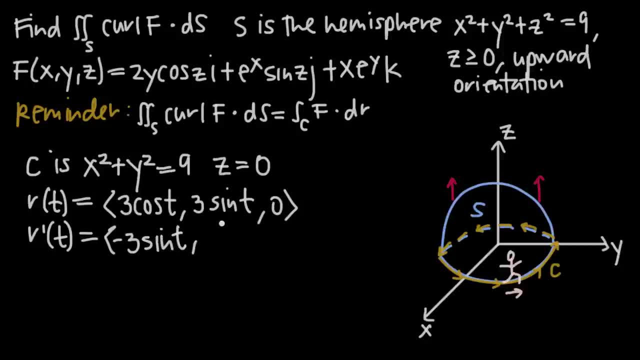 We get negative three sine t. The derivative of three sine t is three cosine t and the derivative of zero is still zero. Now the last thing we need, because we're going to be evaluating this integral on the right with respect to r- we need the vector field f in terms of the vector function r. 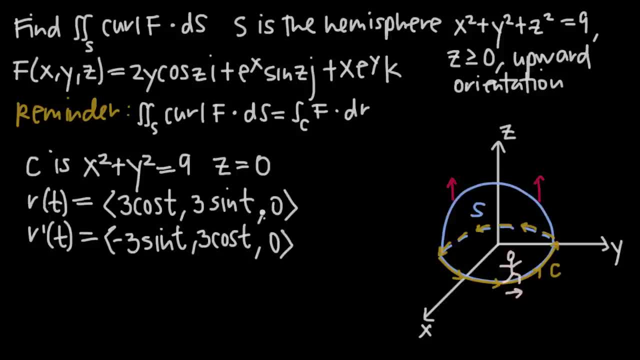 So what we want to do is plug this vector function r into our equation for f of x y z. there then is f of r of t is going to be equal to. we'll take our three values here for x, y and z and plug them into f of x y z. So 2 times y, there y is 3 sine t, so we get. 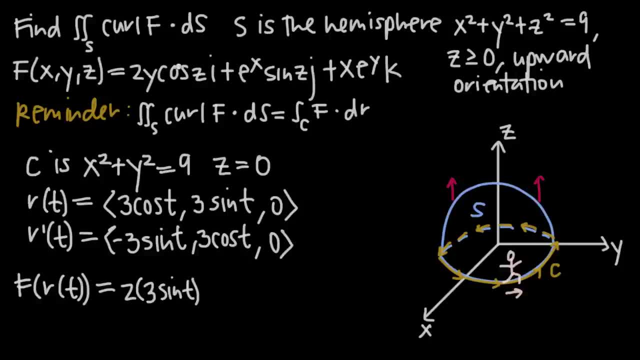 2 times 3 sine t, and then we're multiplying by cosine of z, which is just going to be cosine of 0. Then we want to plug r of t into e to the x sine z. So e to the x is going to be: 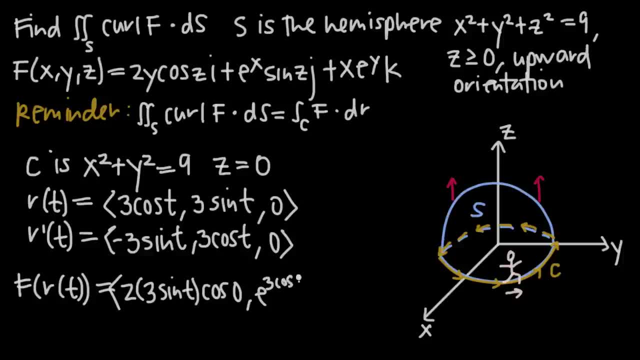 e to the 3 cosine, t times sine of z, so times sine of 0. Then we just need to plug into x e to the y. Let's go ahead and move this out of the way. So because we have x, we'll. 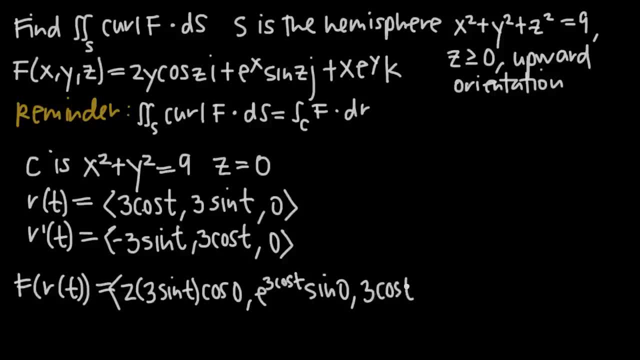 get 3 times cosine of t, so 3 cosine of t, And then we have e to the y, So we'll get e to the three sine t, so three sine t. We want to simplify that. so here cosine of zero is one. 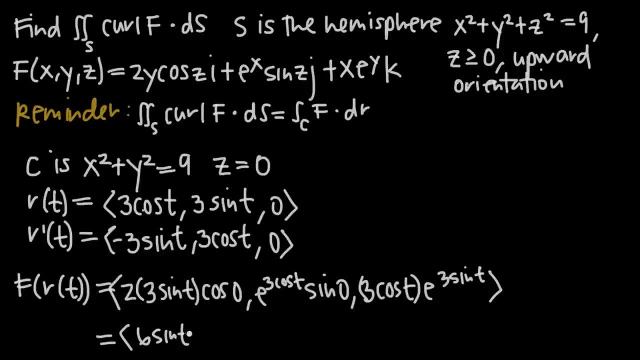 so we're just left with six sine t. Sine of zero is zero, so that whole term's gonna become zero. and then here we can't simplify any further. so we get three cosine t e to the three sine of t. 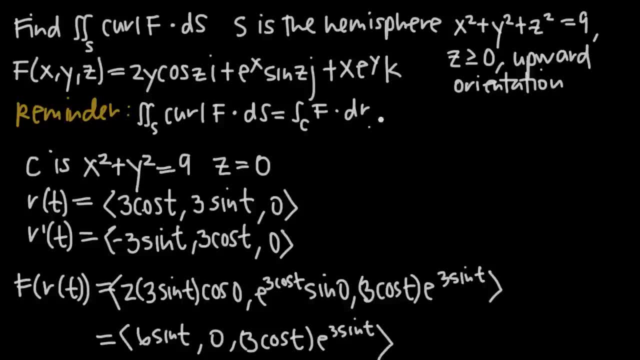 Now, with this information, the integral here on the right-hand side is going to become the integral from zero to two pi, because in fact when we parametrized the curve into the vector function r of t- remember this was the circle here- 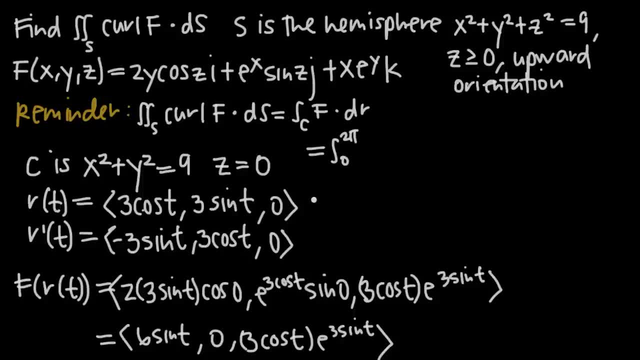 so what we need to do is define t over the interval zero to two pi. so we would say t is the interval zero to two pi. Those bounds get translated here into the interval zero to two pi, which is the integral and then the dot product here. 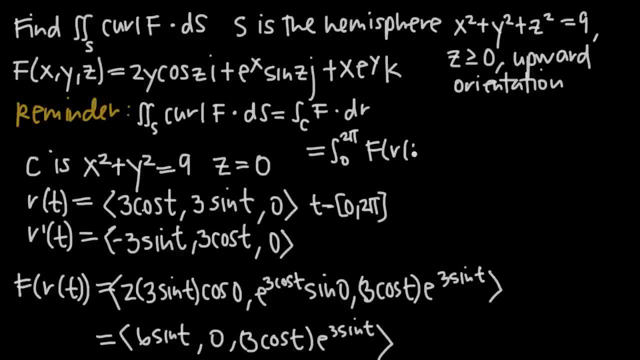 of f? dr is gonna turn into f of r of t, which remember we already found, and the dot, product of the derivative of the vector function r, prime of t, dt. And notice, we already have all of these components so we can just plug them in. 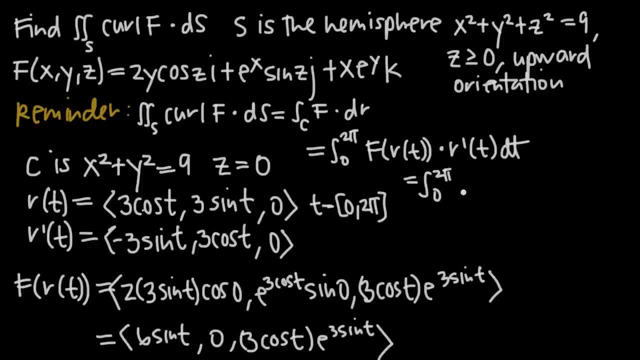 So we'll have the integral from zero to two pi, and let's go ahead and take the dot product now. So we have f of r of t, so that's gonna be this value here, and then we have r prime of t. 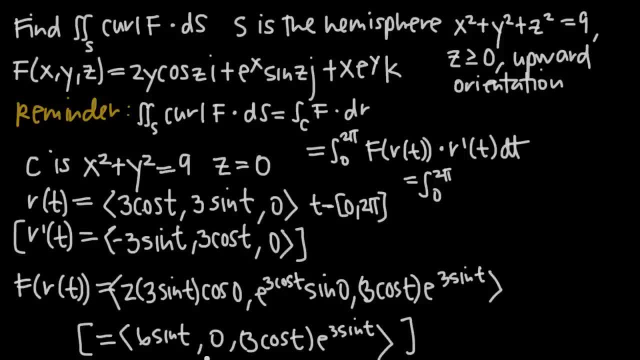 which is gonna be this value here. So we need the dot product of these two, which means we take the x values and multiply them together, then add the product of the y values, then add the product of the z values. So here, when we multiply negative three sine t. 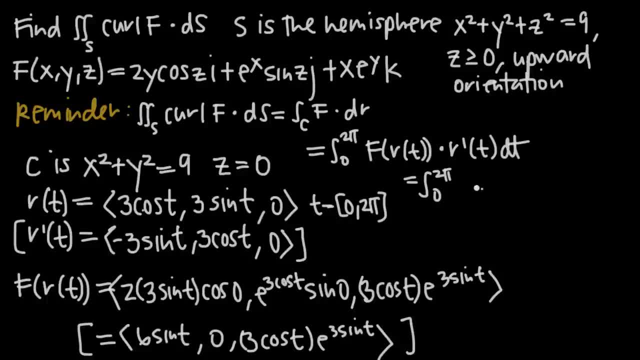 by six sine t, we get negative 18 sine squared t, so negative 18 sine squared of t. Then we're gonna add to that the product of the y values. Well, down here we have y is zero, and then we have t. 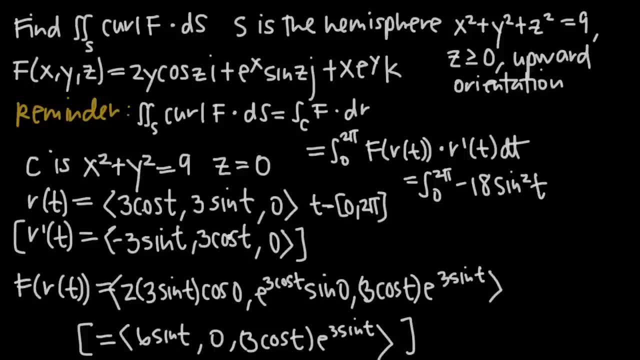 is zero. so when we multiply that by three cosine t, we'll get zero. And here we have z equals zero. so when we multiply zero by three cosine t e to the three sine t, we'll get zero there as well. 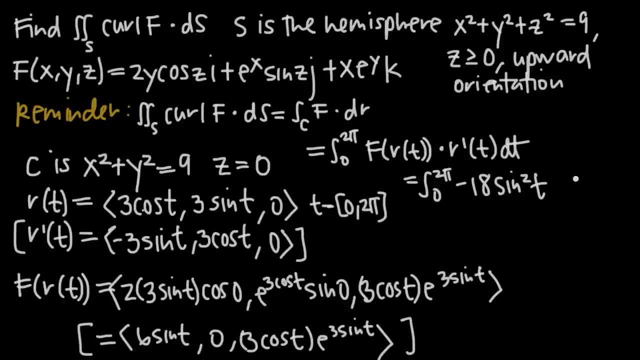 So here we'd have negative 18, sine squared t plus zero plus zero. Obviously we don't need to write those, and so we just have dt. And from here we're just evaluating the integral. We'll make a substitution for sine squared of t. 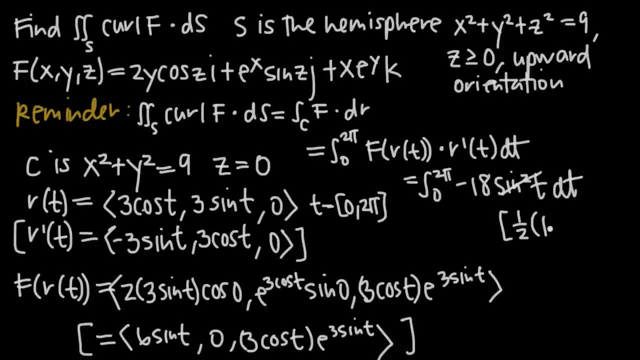 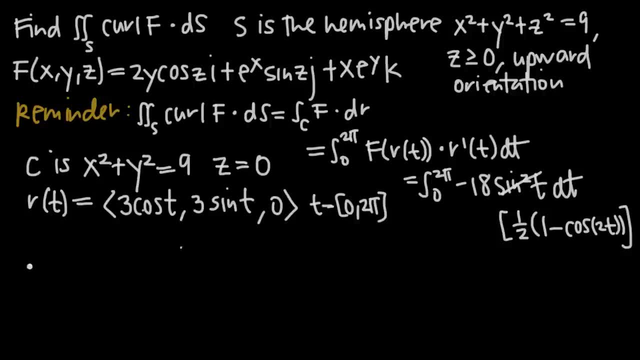 and replace it with one half, which is one minus cosine of two t. And so then, when we grab our negative 18 and our one half, we get a negative nine out in front zero to two pi, and we're just left with one minus cosine of two t dt. 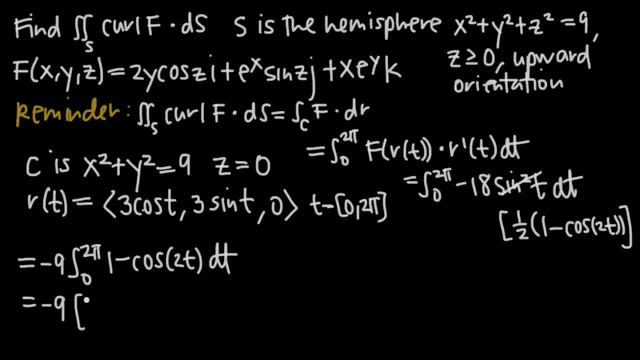 When we evaluate the integral there we'll get t minus one half sine of two. t Evaluated over zero to two pi, When we plug in there we'll get negative nine. And then here, plugging in two pi, sine of two times two pi is sine of four pi. 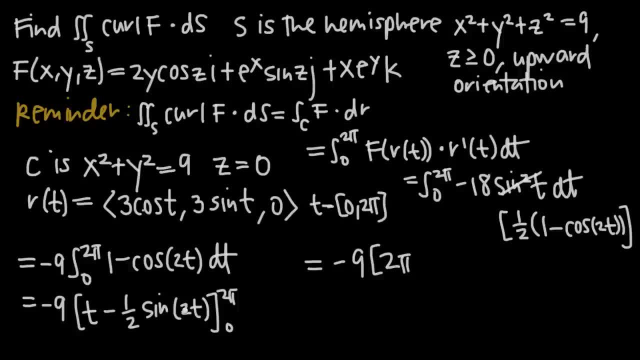 Sine of four pi is zero, so no need to subtract zero there. But then if we go ahead and plug in zero, we'll get zero. here for t We'll get sine of zero, which is also zero. so we really just end up with two pi minus zero. 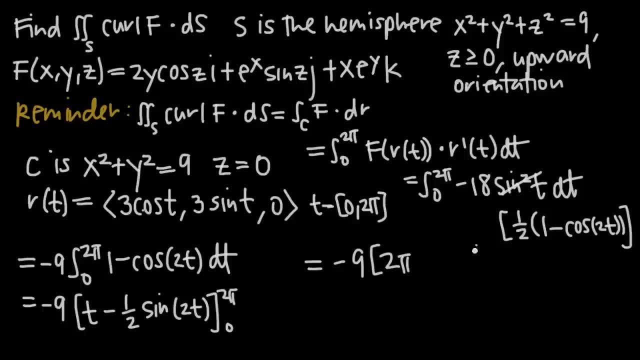 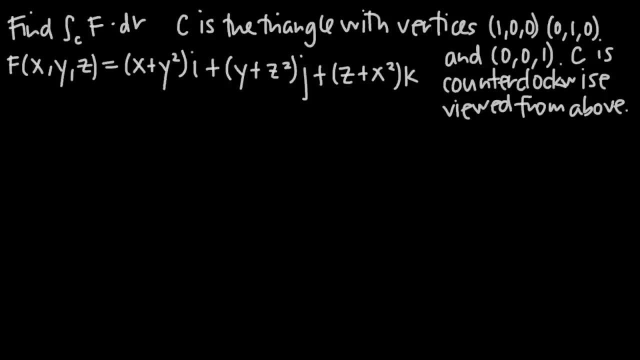 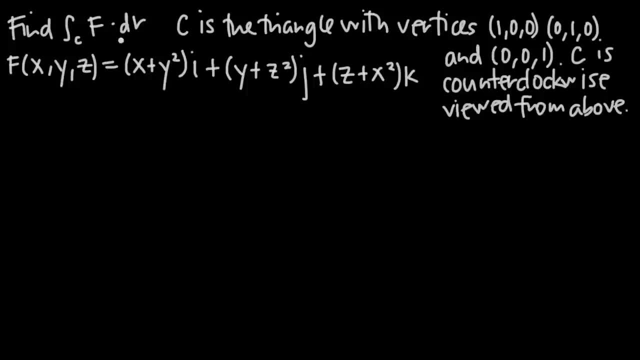 Here we're gonna go the other way with Stokes' theorem. We've been asked this time to find the line integral side of the theorem, which means we're looking for information from the other side of the theorem. We've been told that the curve C is the triangle. 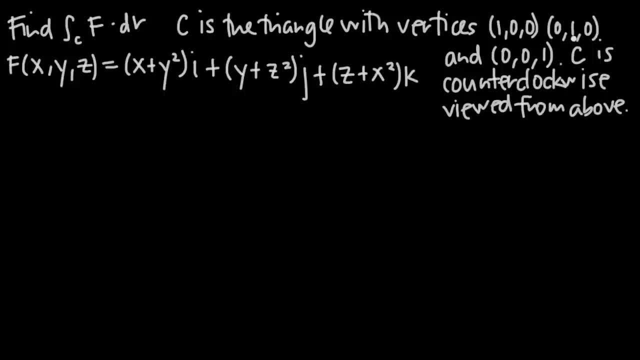 with vertices: one zero, zero, zero, one zero and zero zero one. and that C is counterclockwise when viewed from above And we wanna sketch the surface if we can. Here we're looking at the triangle. 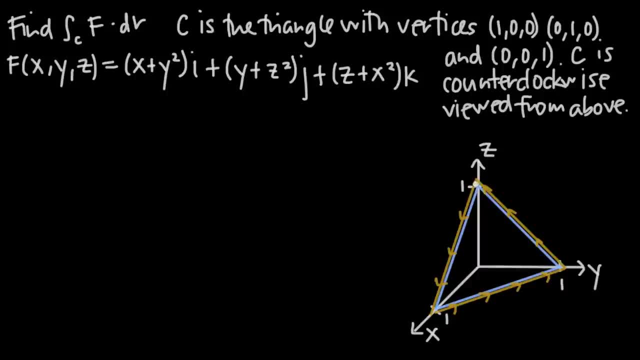 with the given vertices, and we've been told that C is counterclockwise when viewed from above. So again, we're up here looking down and C is counterclockwise, which means we're in good shape, because that's the orientation we want. 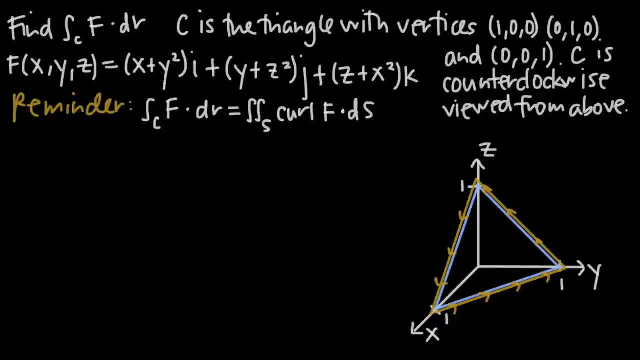 for the boundary curve C. Now remember, we have our Stokes' theorem formula and we've been asked to find the line integral side of the formula, which means we've been given information from the right-hand side of the formula Or we need to find it. 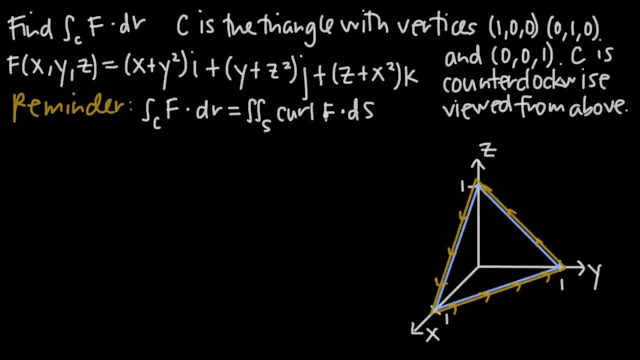 So the first thing we wanna do is tackle the curl of the vector field F. Well, we've been given F here, so finding curl is just an application of the formula for the curl of F. So we'll go ahead and say that the curl of F is equal to. 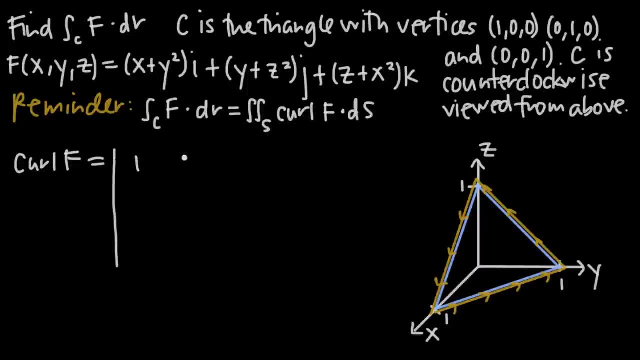 and remember we have our three by three matrix here. We have I, J and K, We have the partial derivative with respect to X, the partial derivative with respect to Y and the partial derivative with respect to Z. This is all gonna be of values from F here. 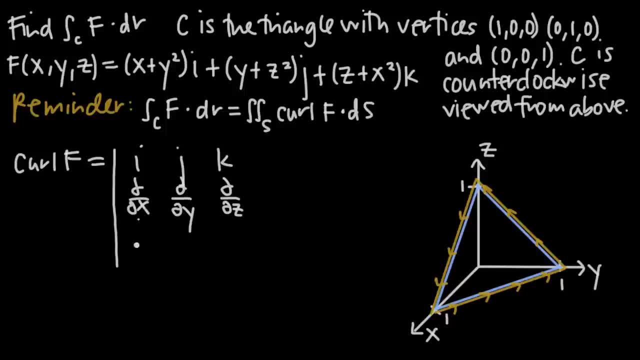 And then we're gonna take X, Y and Z, the coefficients on I, J and K, down here into this third row. So we're gonna have X plus Y squared, We're gonna have Y plus Z squared, and we're gonna have Z plus X squared. 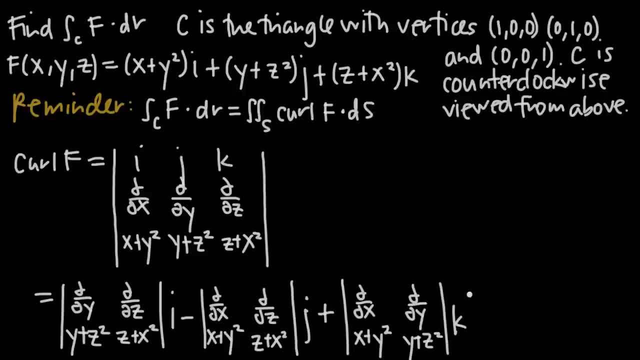 Now remember, when we evaluate this matrix, we're gonna evaluate it this way: We've broken it apart into two by two matrices and now we need to find the coefficients on I, J and K. So here we're gonna say partial derivative. 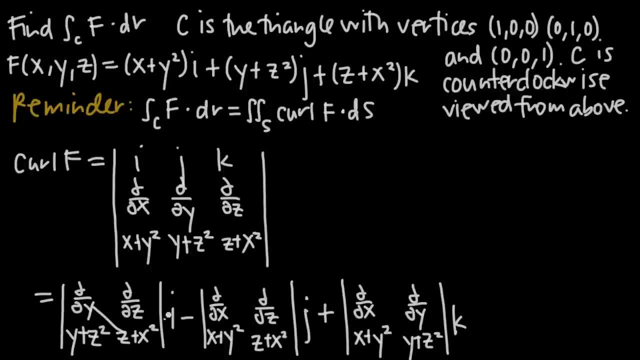 with respect to Y of Z plus X squared. Well, since there's no Y term in there, the partial derivative is zero. Then we're gonna subtract whatever we get when we multiply the opposite way. So here we're gonna say: partial derivative with respect to Z of Y plus Z squared is gonna be two Z. 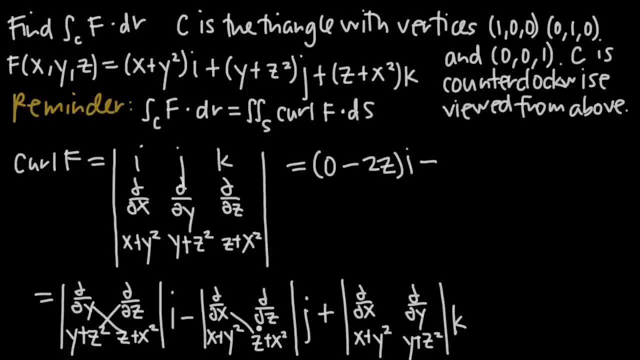 Then for J we're gonna say: partial derivative with respect to X of Z plus X squared is two X- x minus the other multiplication. partial derivative with respect to z of x plus y squared is 0 times j. And then here for k, partial derivative with respect to x of y plus z squared. 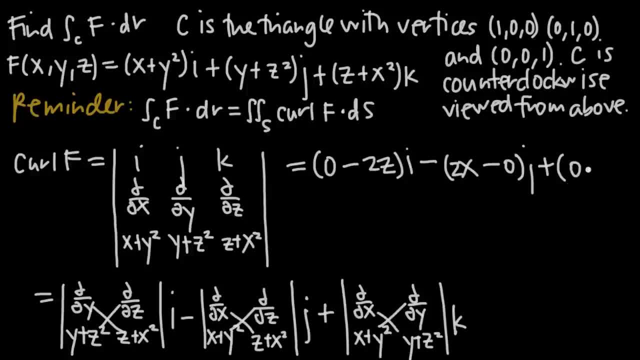 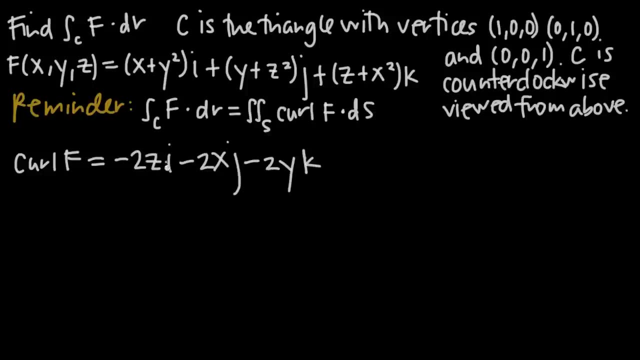 is 0, partial with respect to y. of x plus y, squared is 2y, so minus 2y k, And that's going to simplify to negative 2z times i minus 2x times j, minus 2y times k. Now here's where. 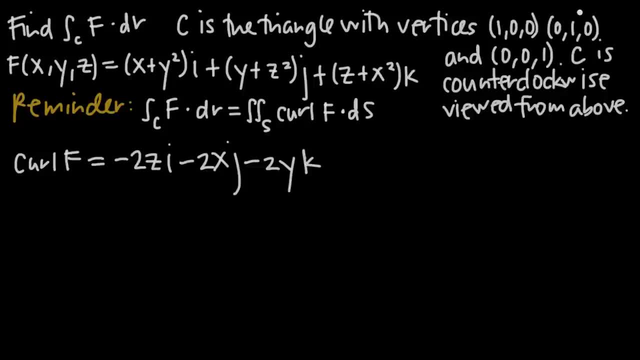 things get a little tricky when we're dealing with something like this, a triangle with these vertices, instead of just the equation for a curve. Here's what we have to do. We have to recognize that curl f is given by p times i plus q times j plus r times z. So 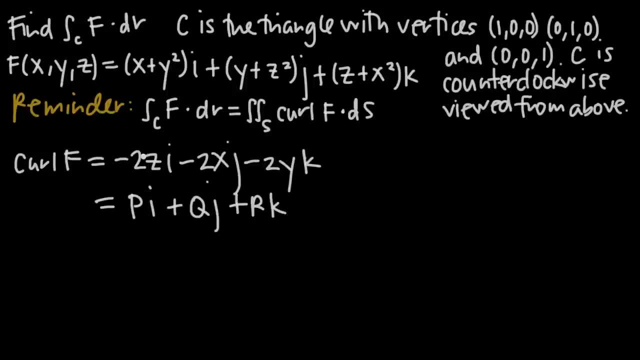 this is k, And so then what we want to say is that p is equal to negative 2z, q is equal to negative 2x and r is equal to negative 2y, Then what we know is that this value we're. 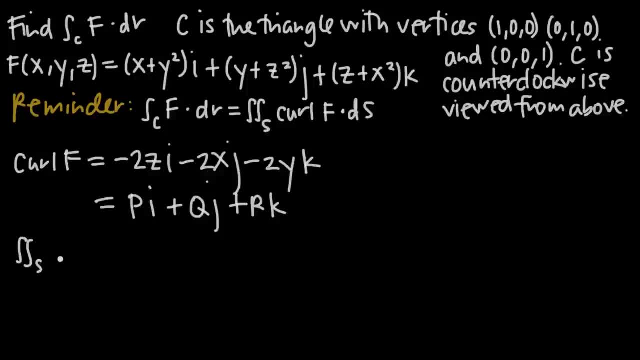 trying to find here this right hand side, the double integral over the surface s curl f, dot product ds that that's actually equal to the double integral over d, where d is the projection of this surface. we're interested onto the xy plane. We'll come back to that. 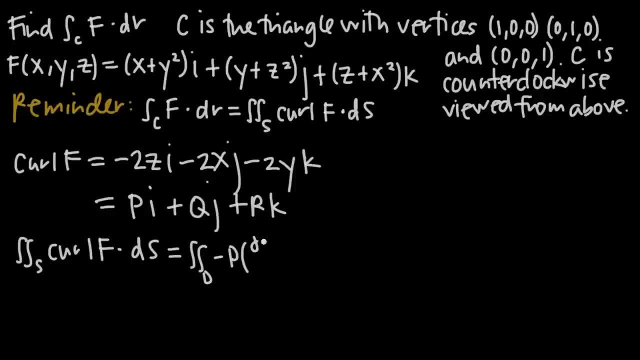 in a minute Of negative p times partial derivative of g with respect to x- and we'll come back to g in a second- minus q times the partial derivative of g with respect to y, plus r times dA. Okay, so we just threw a lot out there. We already know p, q and r. they come from the value. 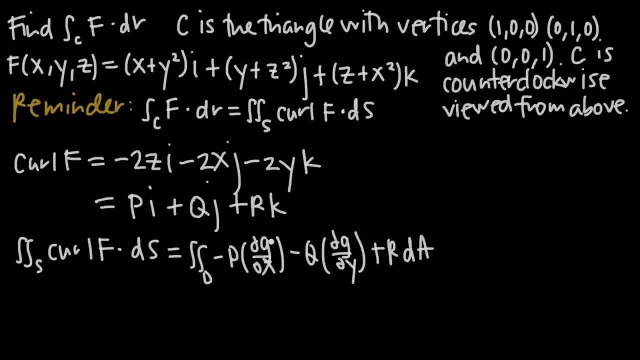 we just found for curl. But what's this function g? Well, g is going to be the surface, the plane that we're interested in. Remember we looked at the surface, the plane that we're interested in. Remember we looked here at our triangle. This surface is going to be part of the plane. x plus y plus z equals. 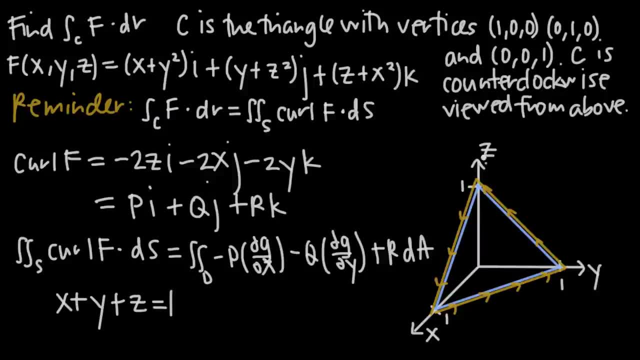 1. This plane right here is the plane that intersects the x, y and z axes, all at x equals 1, y equals 1, z equals 1. So this surface is part of this plane. If we solve this equation, 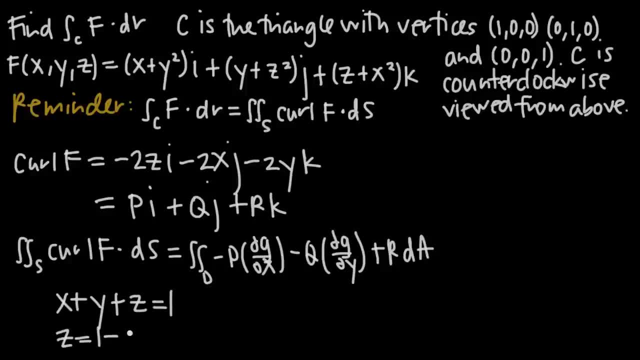 for z we get: z is equal to 1 minus x minus y. Now that we have z as a function of x and y, we can just rename this and call it g of xy. So we'll say g of x- y is equal to 1 minus. 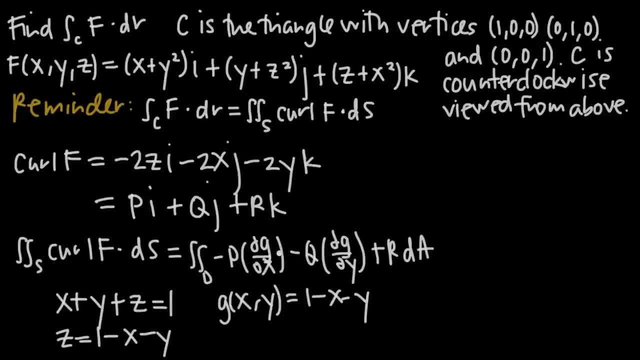 x minus y. Now this function, g, is what we're talking about when we're saying the partial derivative of g with respect to x and with respect to y, So we're going to be able to easily find those. We already have p, q and r, so all we have to talk about here is this: 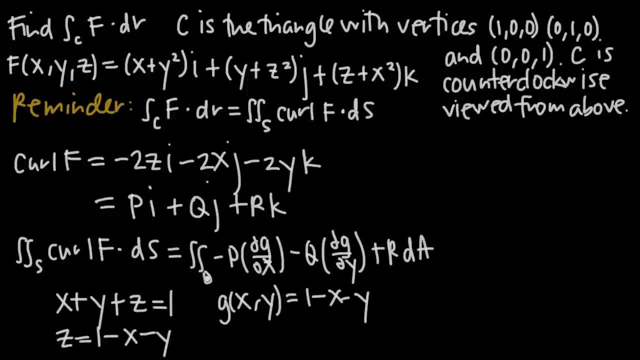 d, And remember we said d was the projection of the surface onto the xy plane. Well, if we go back to our picture here and we think about this as the plane intersecting the coordinate axes at x equals 1, y equals 1,, z equals 1, and we just think about what shadow it would, 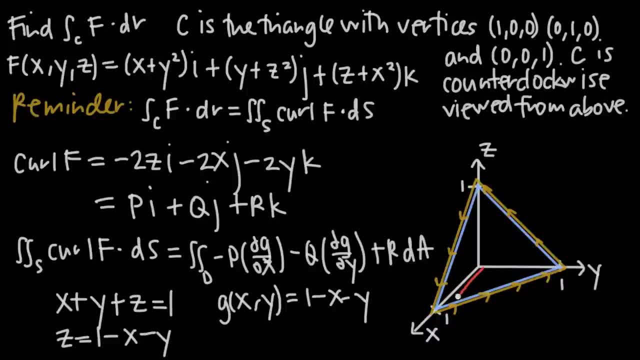 create on the xy plane. its shadow would be this little triangle right here, And this little triangle would have the vertices this would be and this would be, And that'll be the projection d, And we'll come back to that in a second. For now, though, because we're trying to find this, 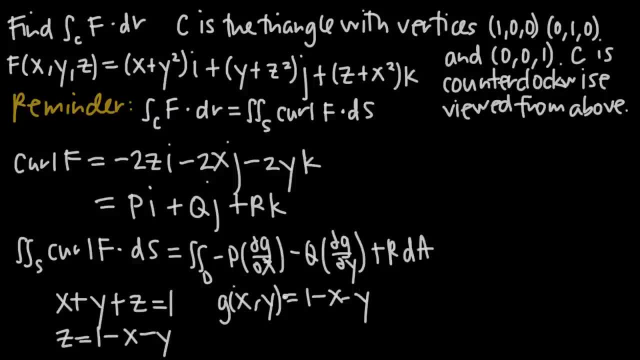 double integral over the surface s. all we have to do is plug into this double integral over here on the right. So we'll go ahead and say that that's going to be equal to the double integral over the region d. Here p, we already know, is negative 2z, so we're going. 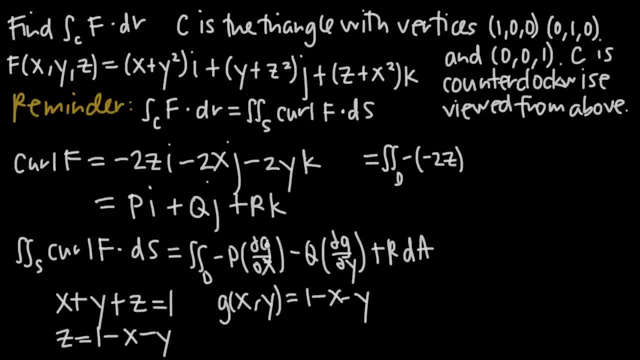 to have negative: negative 2z times the partial derivative of g with respect to x, which is going to be negative 1.. Then we have minus q, which we know is negative 2x times the partial derivative of g with respect to y, which is negative 1.. And the plus r, which 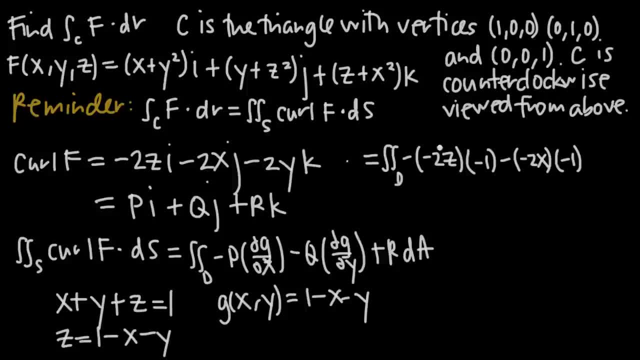 we know is negative 2y, so plus a negative 2y, so we have minus 2y and we have d. When we simplify that, what we get is we have three negative signs here, so that's going to end up as two z. We have three negative signs here, so thats going to end up as a negative 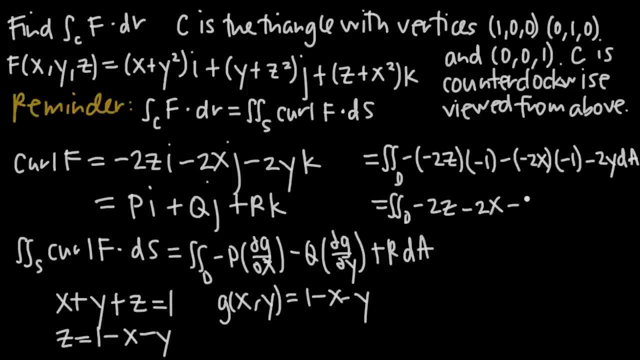 2x And we have a minus 2y, So they're going to be negative 2x times the cross relation E75. for x, we have x. it's going to end up as 2u, So that's going to end up as y And 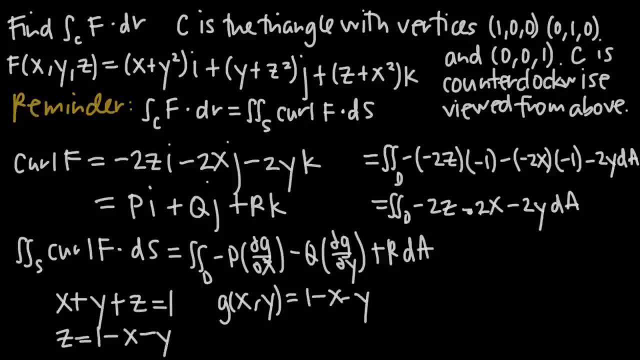 we'll come back to that sub that earlier in the 2nth question. we also have this double dA. We want to then make a substitution for z. Remember that z was 1 minus x minus y. So we're going to get double integral d When we multiply this negative 2 by each term here. 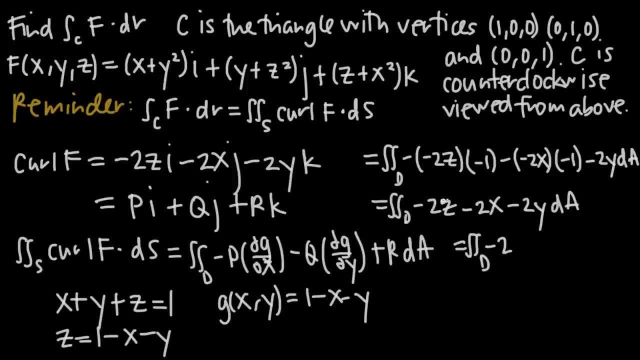 we're going to get negative 2 times 1 is a negative 2.. Negative 2 times a negative x is a plus 2x, and negative 2 times a negative y is a plus 2y. Then we have minus 2x, minus. 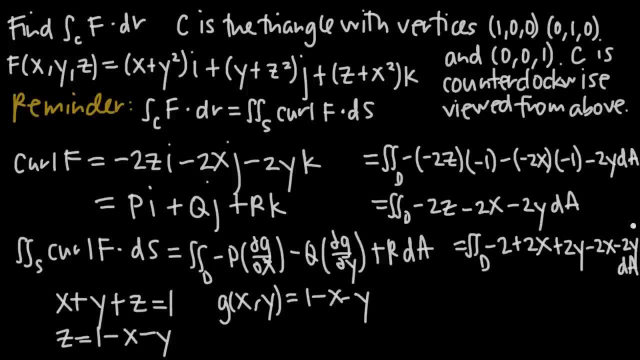 2y and dA. Now notice that we have a positive 2x and a negative 2x, a positive 2y and a negative 2y, So all we're left with is double integral over the region d of negative 2 dA. 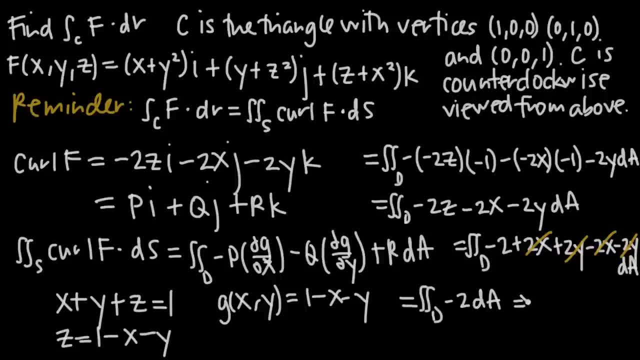 And we can go ahead and factor the negative 2 out of that. so the result then is negative 2 double integral over the region d of dA. And this is where this method really gets cool, because this double integral here is going to be equal to a plus 2x minus 2 dA. 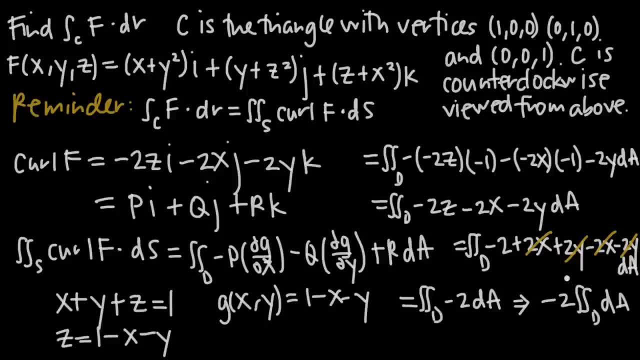 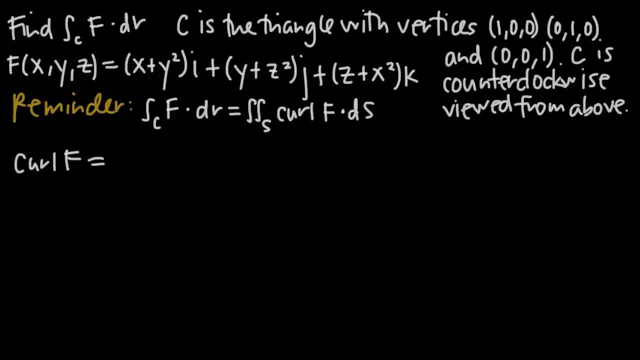 here, over the region D of DA. In fact, this whole thing right here just means the area of that projected region, that shadow on the XY plane. So if we go ahead and bring back that area, we're talking about this region D right here, this shadow, So that thing that we boxed then, this here, this is just the area of that. 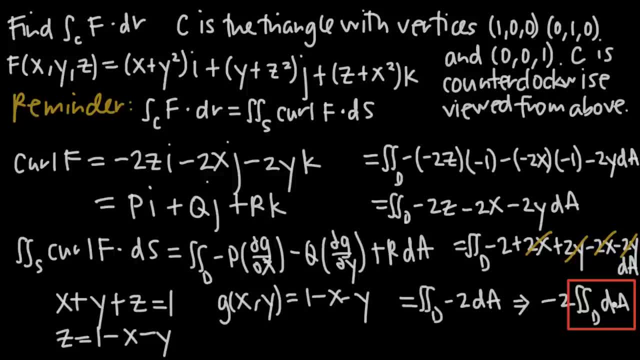 region. Well, remember that region was a triangle with side lengths 1, so it was a 1 by 1 triangle. The way to find area of the triangle is 1 half times base times height, or 1 half times 1 times 1, which of course is just 1 half. so the area of 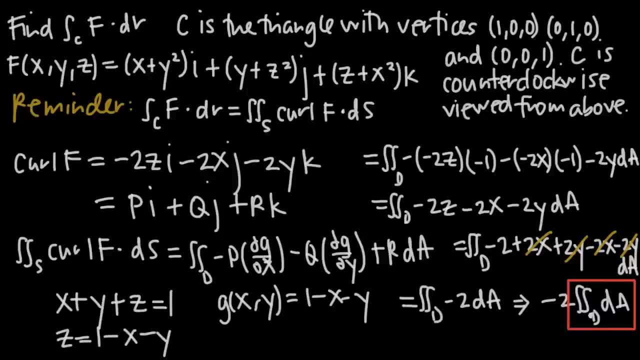 that shadow, the area of that projection, is 1 half, so this whole thing is going to become 1 half. So our result then is going to be equal to negative 2. this negative 2 here times 1 half the area of that region, and negative 2 times 1 half. 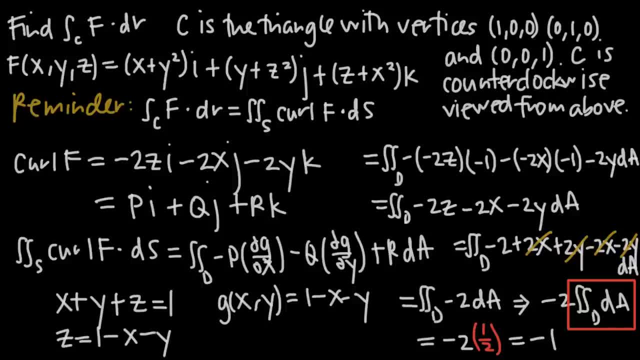 is just going to be equal to negative 1. you.